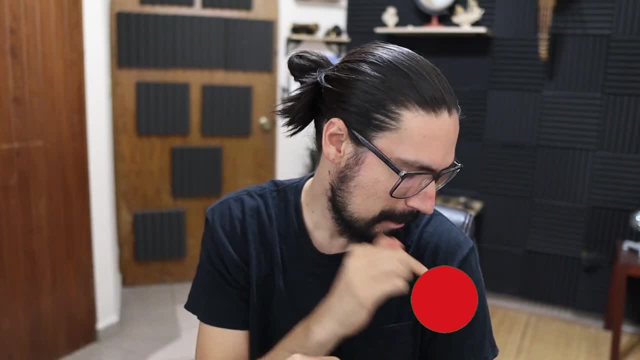 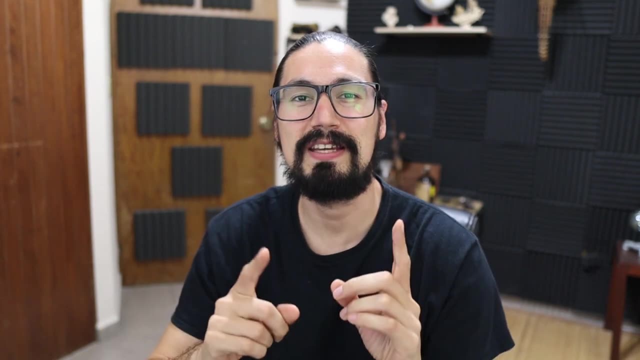 usa. so don't hesitate and click on the notification bell right here so you get all my latest video specifically on this video series. so now that you know this, let's get started. okay, guys? so just in case you are not quite familiar with the linkedin search, 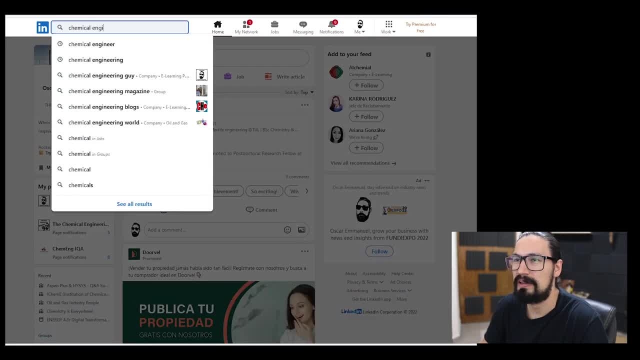 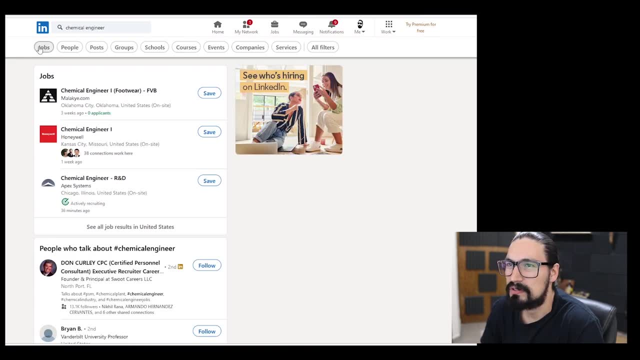 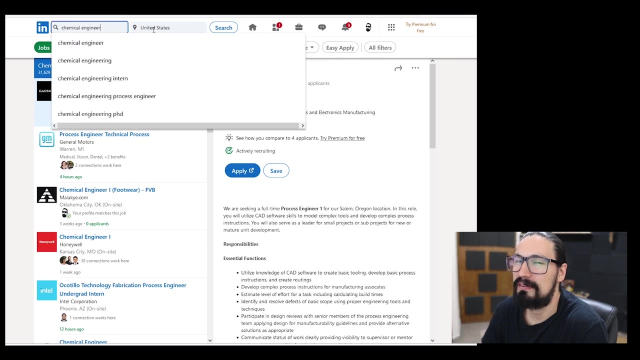 i'm going to be searching here for chemical engineer and, as you can see here, there are several options in these tabs. i'm going to be searching for jobs. okay, depending on how you search, you will have several pre-filled, or, let's say, default selections. right now i'm going to be searching for chemical. 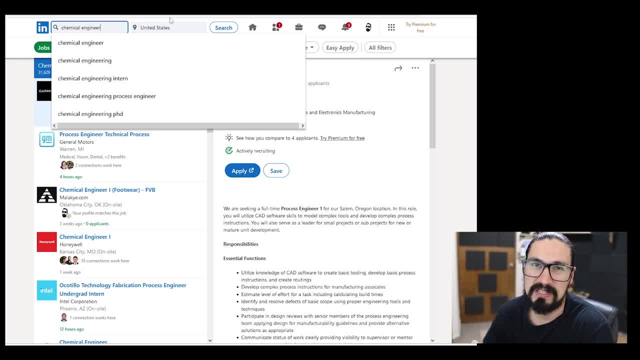 engineer or chemical engineering. you can do the same for process engineering or anything related towards chemical engineer, and i will be searching for united states right now in this specific video. not only that, guys, i want to be a little bit more picky, because we have 31k. 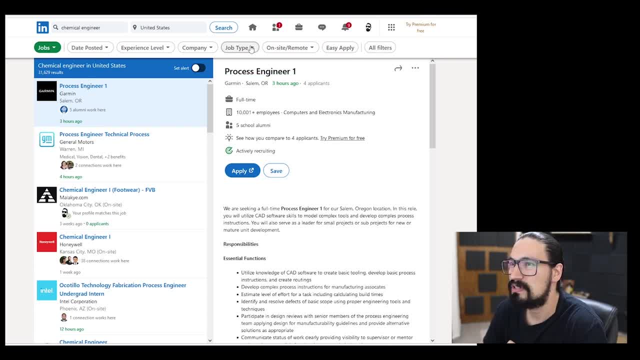 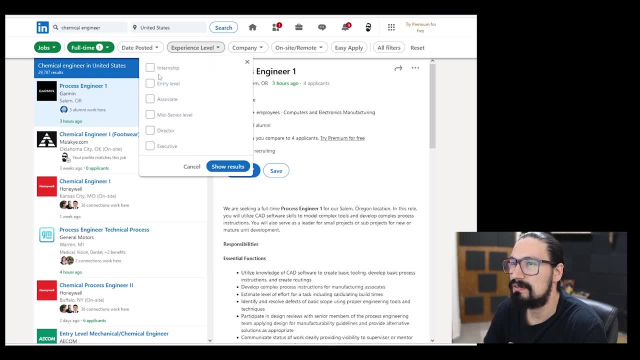 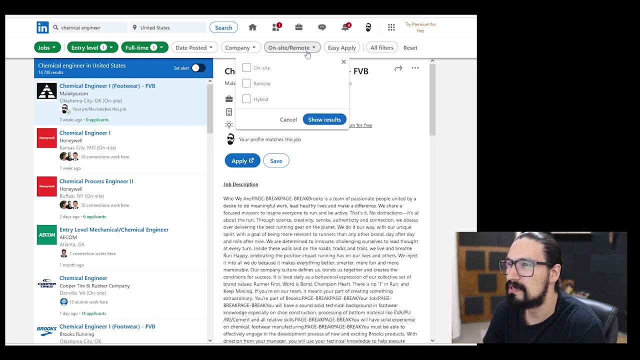 results, which is a lot. so first things, first. job type: let it be a full, then. i want this to be a entry level job. for a reason: graduate, most likely. i'm not going to be picking on companies on site, remote, well, most likely going to be on site, but let's say we are. 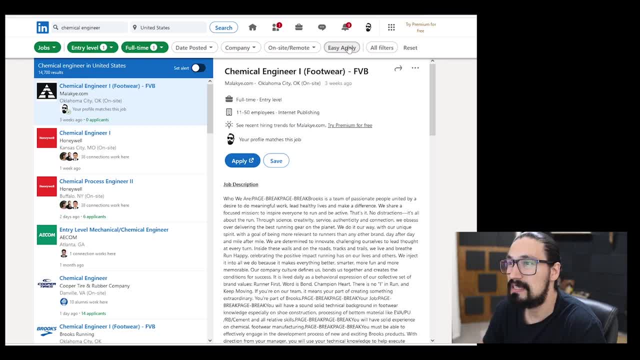 open for this easy applies. the easy apply, essentially an option that allows you to apply directly via linkedin, is very easy for the linkedin application. so for the linkedin application and the on the linkedin page and if you go into the architecture website, let me get a view of the linkedin. in course with eahi. effectively, for example, linkedin provides you with existing startups and which can you jadi up? how they offer up, how they offer them for해서 the list there. is there some things where you can use the e a play here and then take some choices. in this example, we have a sucks for options. 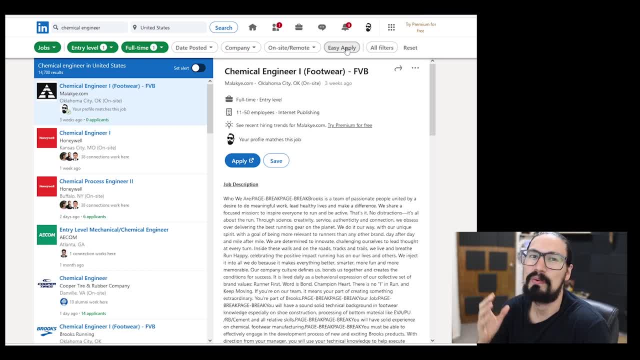 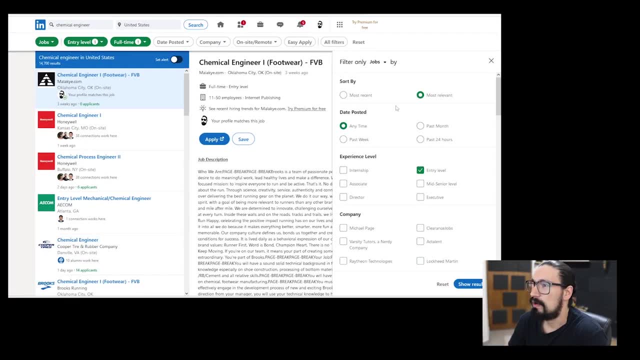 the LinkedIn user both ends the recruiter and the one searching for a job. but not many jobs do that, so I'm not going to do that. All filters, so right now I'm going to be searching overall the options, but, as you can see, the most interesting part is right. here: 40k, 60k, 80k, 100k, 110k. actually I'm kind of curious to see how much. we have almost 15k results. so there's only 252 jobs that offer a 100k plus per year. 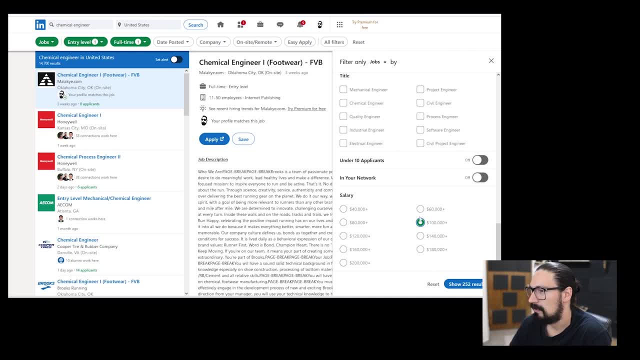 salary, which should be something very, very low. 80 should be something more feasible, 1000, and remember guys, this is entry-level jobs, so I will aim something in between 60 and 80, so you can see, 60 is 5k. yeah, makes much more sense. 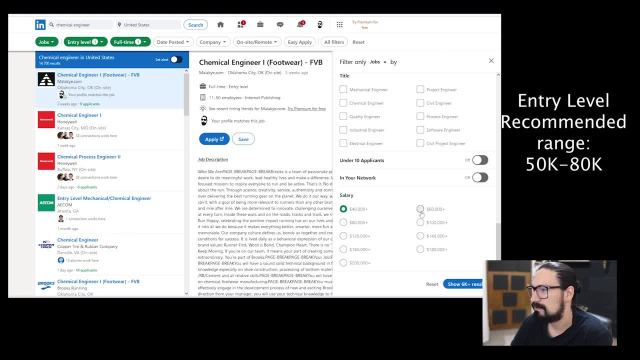 40k, 6k. so we have 6 plus 5, 11 plus 1, 12, well, it doesn't match up, but essentially you should be aiming something between 60 to 80.. Right now I'm not going to be analyzing that, let's ignore this. 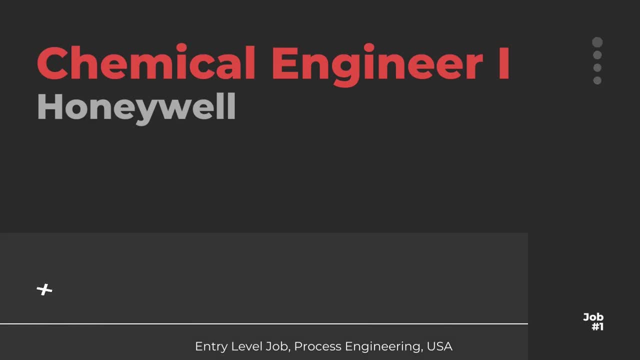 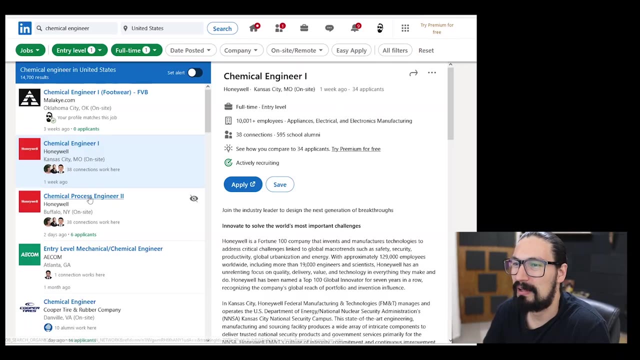 and quickly. let's get started. Chemical engineer 1, not quite sure what does 1 mean? probably entry level 1, or, for instance, we have chemical process engineer 2, I don't know if these are several options or maybe it's. 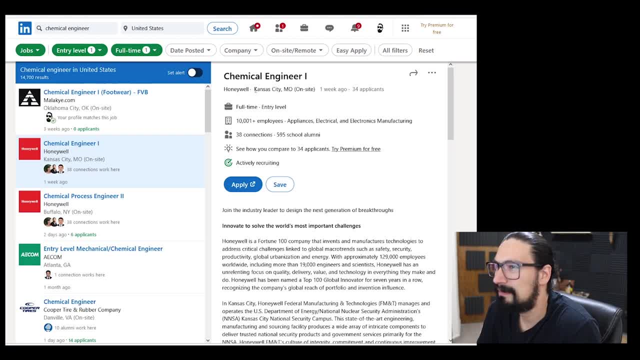 Maybe it's a level within the company, so just keep that in mind. Honeywell, very known company always. you can check out here if you want to learn more about the company. but right now let's stick to the actual job: full-time, entry-level, my connections and how many of my classmates have 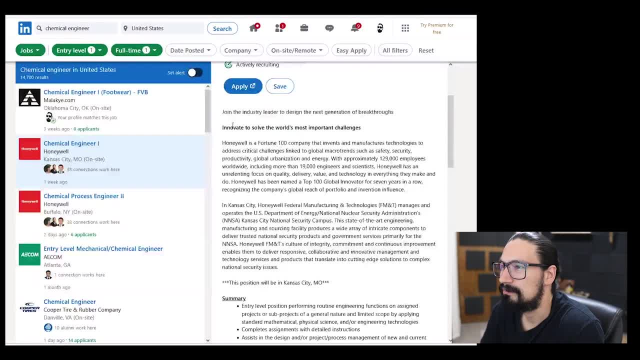 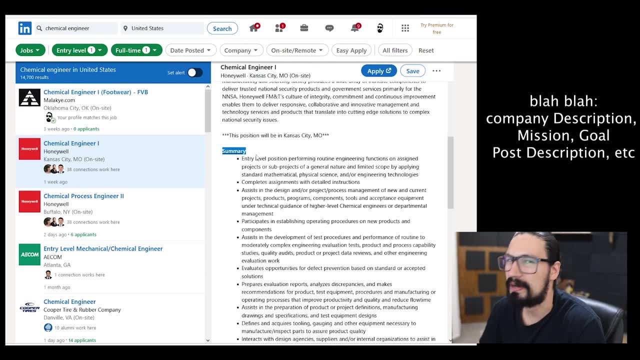 been working there and let's go. Okay, so this is almost the blah, blah blah of the company. what you want to go is always to the summary. What are you going to put into the summary If you're nothing? if you're looking for a job or you have a degree. if you're not a degree, you're going to have to get an. 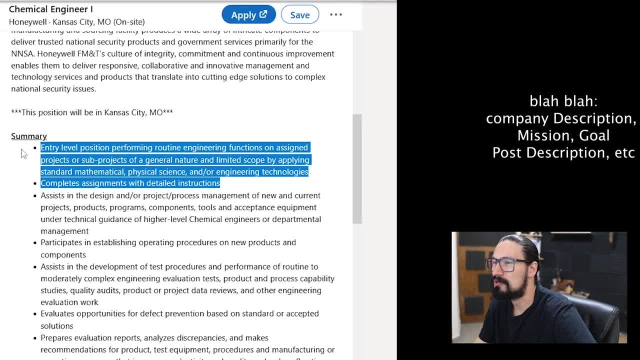 are you going to be doing? Clearly stating entry-level position: performing routine engineering functions on assigned project or sub-project of a general nature. unlimited scope, by applying standard mathematical, physical or engineering technologies. So clearly this is very broad. doesn't exactly say what you're going to be doing. completes assignment with detailed instruction. 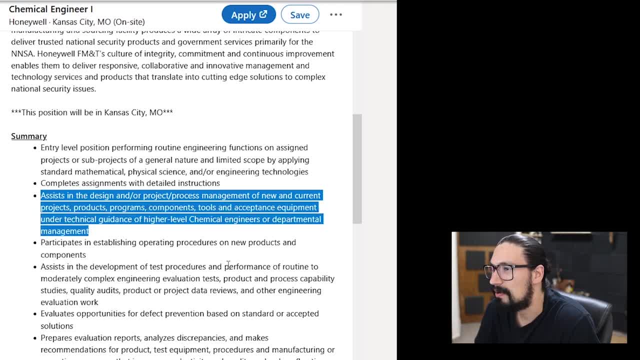 very broad assist in the design and project process, management of new and current projects. okay, this sounds like almost an engineer assistant to an actual engineer, but it's okay because you are an entry-level engineer and this way you can learn more about this Higher level chemical. 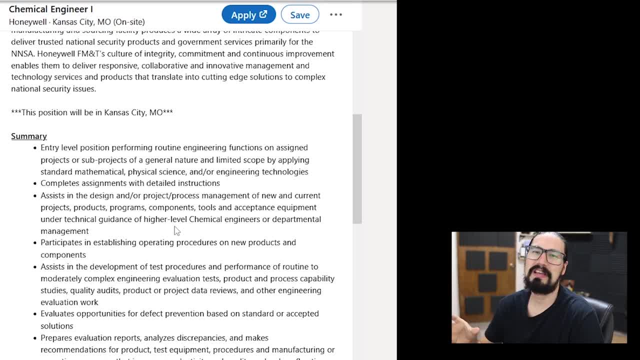 engineers. okay, yeah, exactly what I was telling you. So this is a glorified way to tell you that you're going to be almost an assistant of a actual high-level chemical engineer, which has no problem because, remember, you're going to be doing a high-level chemical engineer. you're going to be 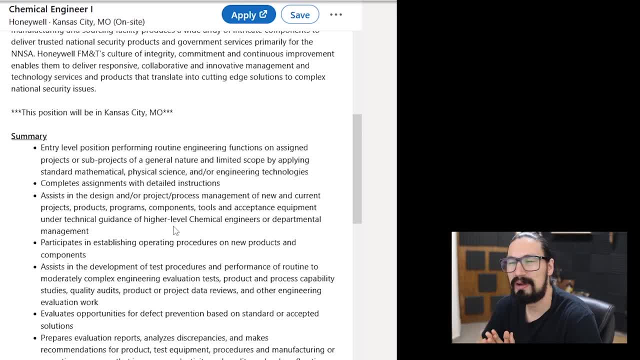 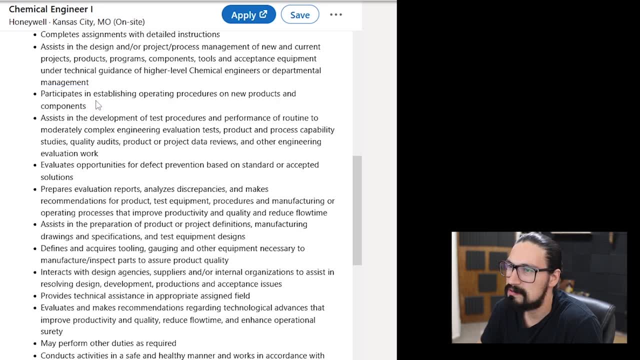 doing a high-level chemical engineer. So remember, guys, you are not an actual chemical engineer. you just graduated right now. you don't know that much about chemical engineering. Participates in establishing operating procedures on new products and components- sounds interesting. Assists in the development of test procedures- okay, that sounds, sounds nice. Evaluation of tests. 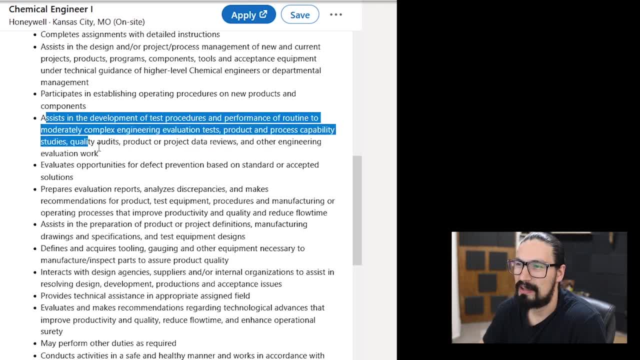 product and process capabilities. This actually sounds great. this sounds like actual engineering job. my main question will be: are you are going to be actually doing that or helping in doing that? I mean many times. let's get honest, guys. engineering requires a lot of just. 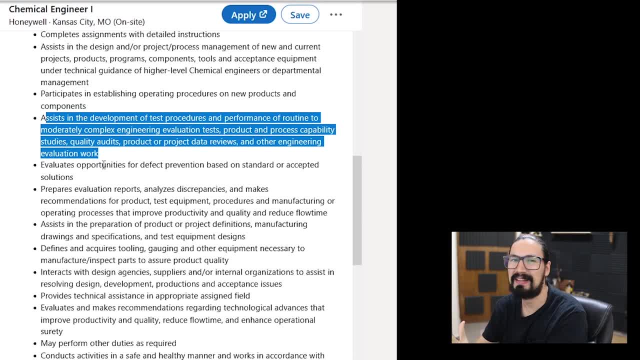 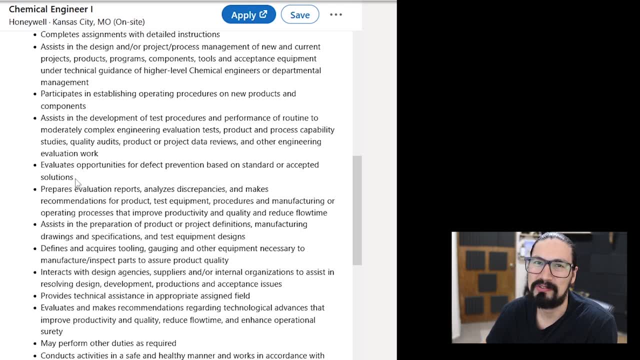 manipulation of data, getting the data, applying that data, getting the data and all that which sounds great when you talk about it, but it's actually kind of boring just to implement those data and read the data. Evaluates opportunity for defect prevention based on standard or accepted. 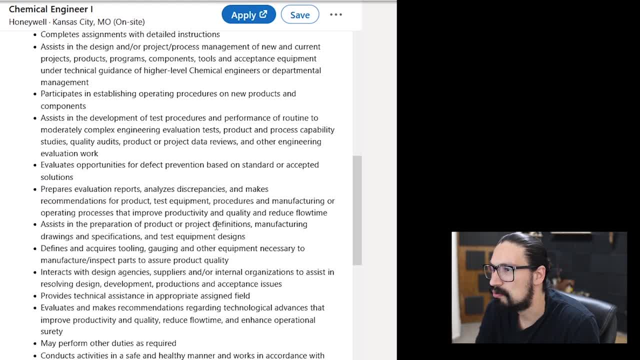 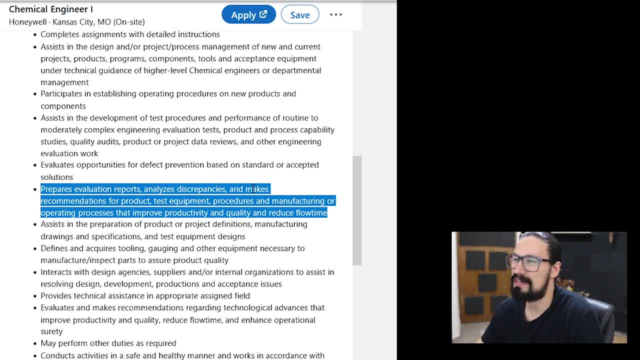 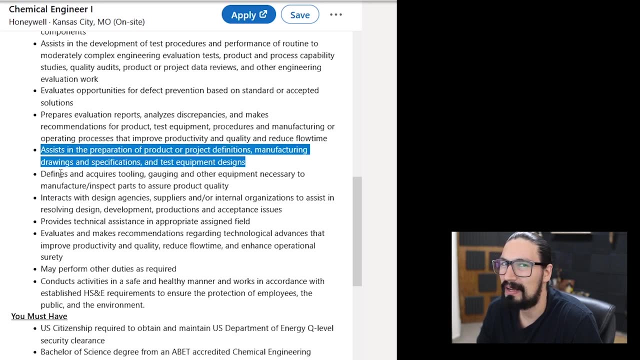 solutions very, very broad. Prepares evaluations and reports, analysis discrepancies. okay, this sounds interesting: actually making reports. making reports is going to be classical process engineering all the way: Assist in the preparation of products, off-project definitions, drawing specifications. this sounds also like actual engineering job: Defines and acquires. 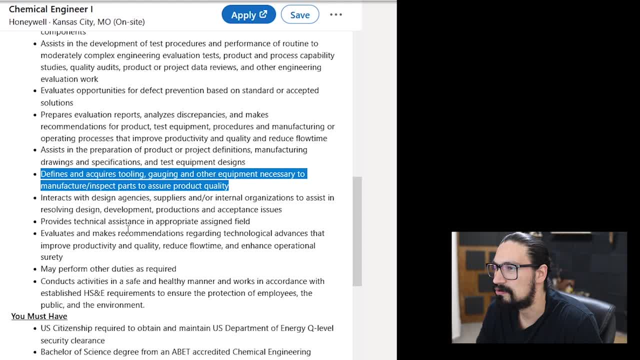 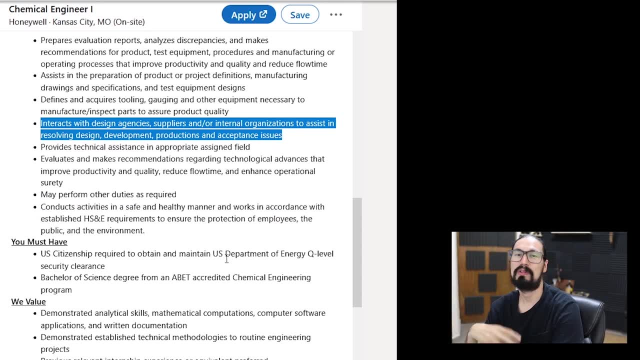 tooling, gauging and other equipment necessary to manufacture, inspect parts too. okay, yeah, Interacts with design agencies. okay, this is great. you are actually interacting with other people, not along with your boss, let it be, or the high-level level chemical engineer. You're going to be interacting with agencies, suppliers, internal. 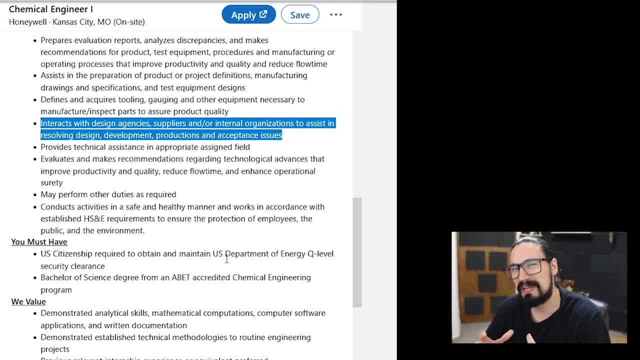 organizations. And this is very interesting, guys, because this may be actually great in the sense that you're actually leading, communicating and getting all this information, Or it may be a very boring process in which you need to call insistently. So this is very hard to say. if it's. 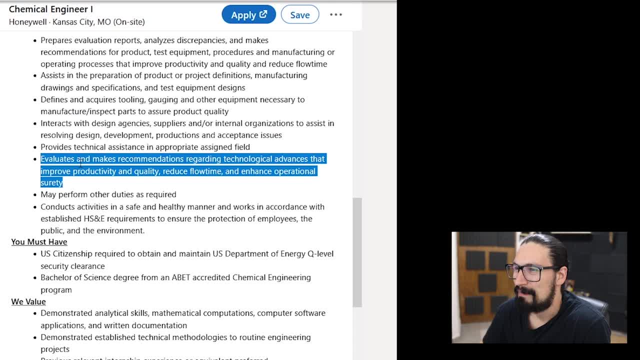 actual engineering job or not, but so far looks great, Provides technical assistance, sounds very great, unless you're actually like a teleperformance or someone in telecommunication, just like telecom guy, trying to fix everything via just telephone. It's kind of boring And, believe me, 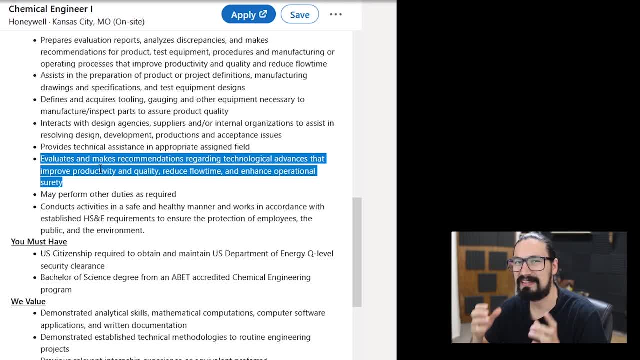 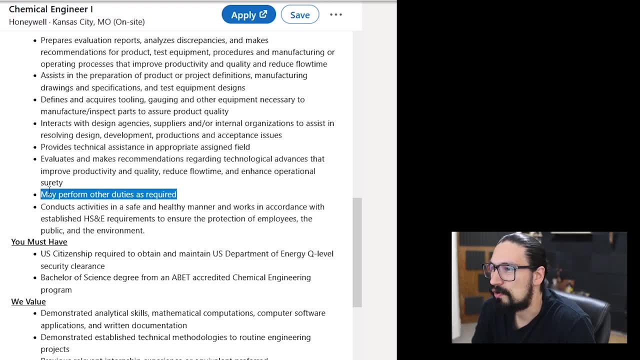 guys. I know process engineers that are actually just doing that. They say they're in technical sales or technical solutions and they are just there chatting via phone and it's not that nice. May perform other duties as required, Okay, yeah. well, this is classical one. At least they are. 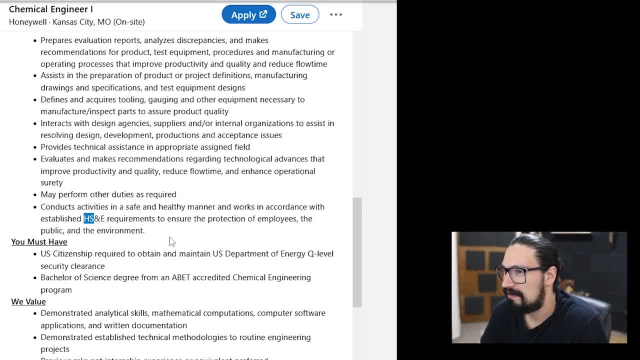 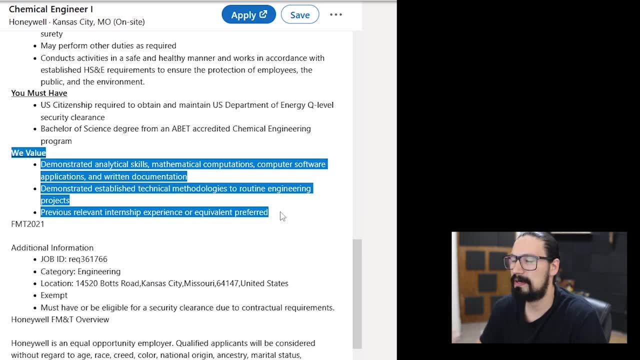 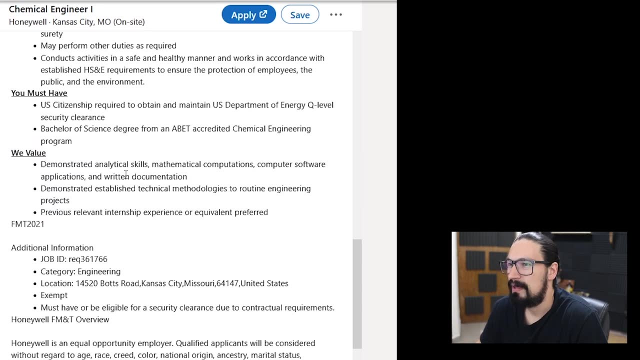 writing it And conducts Healthy, safe and environment stuff. Well, that's also classic: You must be US, We value. So this is the interesting part right here, And actually I have a video on actual skills that employers look for. So definitely go and check it out, But for now they value analytical skills. 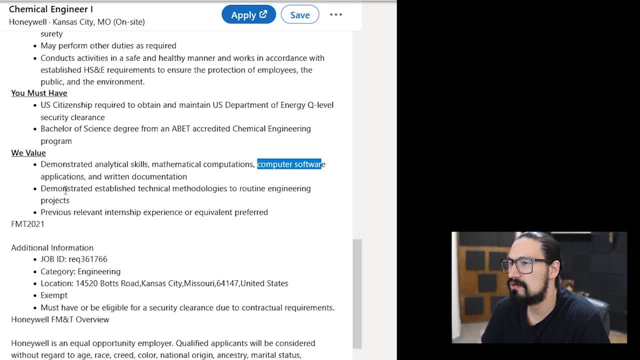 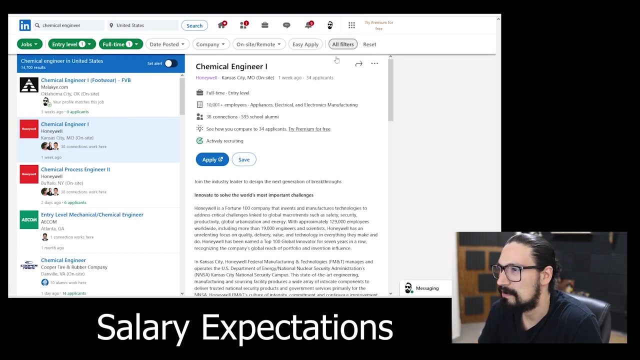 mathematical computations, computer software applications and written documentation, Also technology methodologies and routine engineering projects. So overall complex problem solving, troubleshooting, mathematical skills and analytical skills. And location: Kansas City. So one way to identify how much they are offering is simple: Go to this. 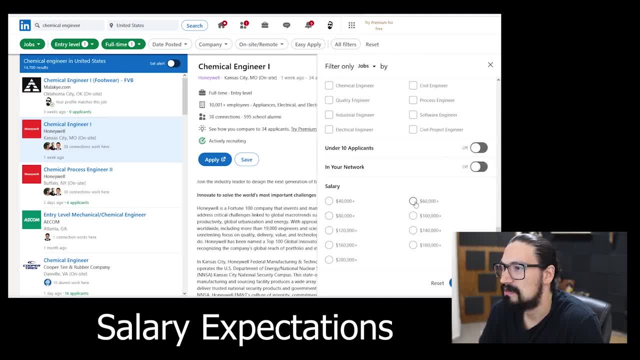 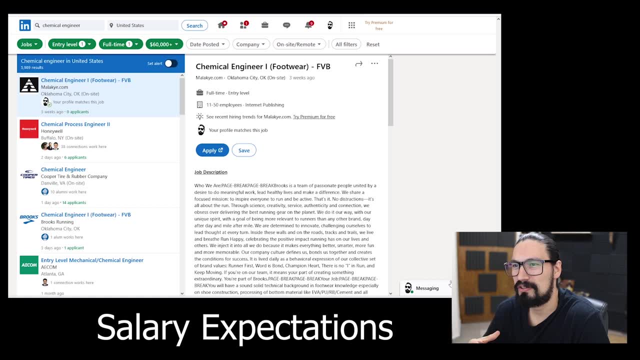 filter and click. Let's assume this is say 60 plus, So you can see the job is not showing. So definitely must be something lower. Maybe higher, let's see. No, definitely lower. So yes, it's between 40 and 60k. So it sounds like you're going to be an engineering assistant for a. 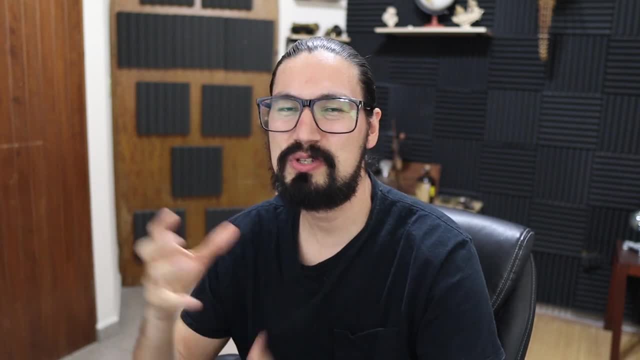 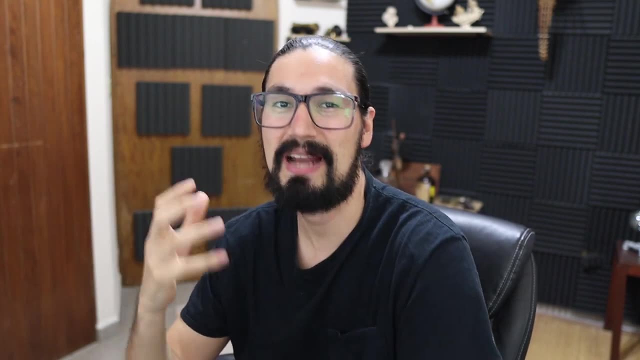 process engineer. You're going to be learning a lot. My main question will be: how stagnant is that job? Are you likely to find another job within the company? How is it likely to you to actually climb the ladder? Is it a ladder? at least, That's up to you guys. 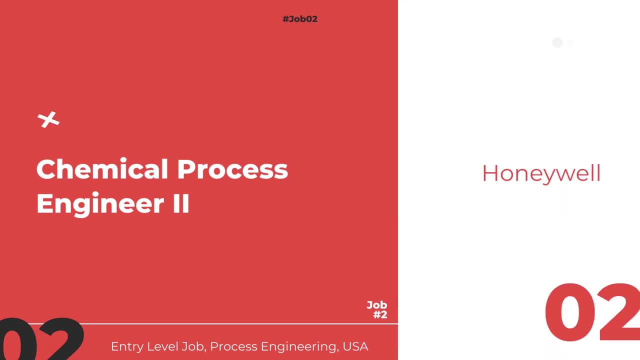 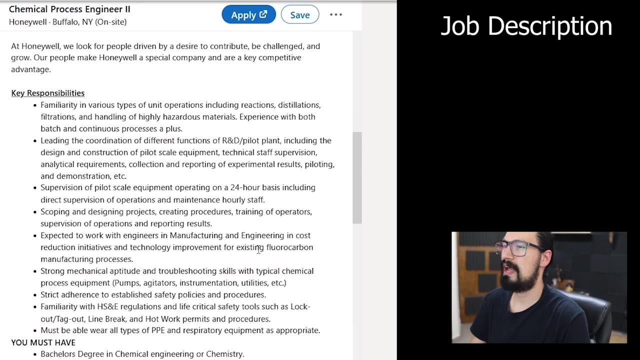 For the sake of this video, I want to check out this chemical process engineer, Same company. but let's go and check out the actual key responsibilities: Familiarity in various types of unit operations, including reaction. Okay, so right away you are getting to the hot. 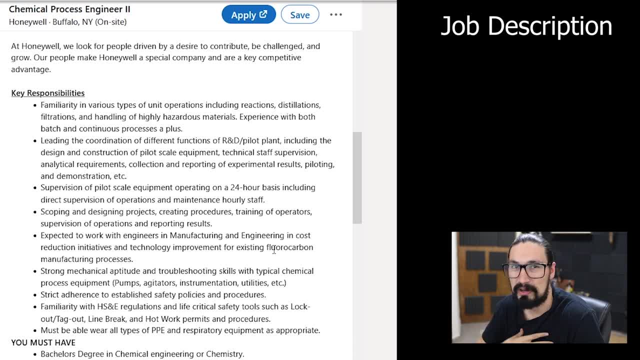 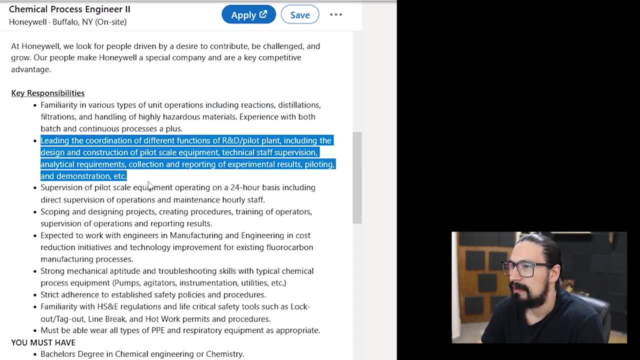 stuff. So definitely this is way better job than the previous one, in my opinion. if you're looking something towards process engineering, Okay, you experience with both batch and continuous processes is a plus. Leading the coordination, So right away you're getting this. 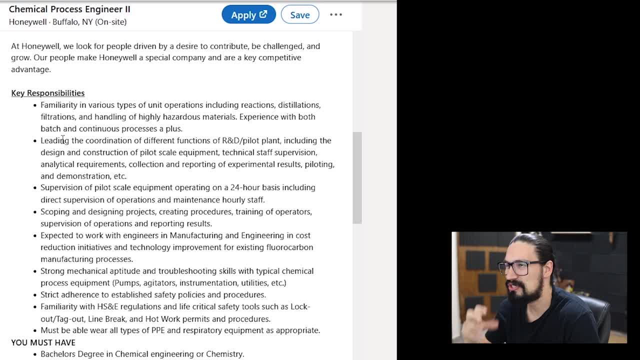 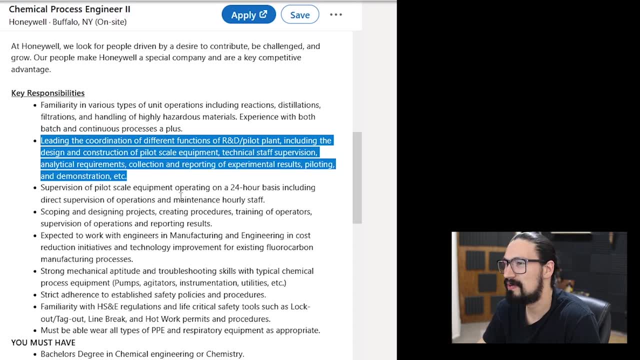 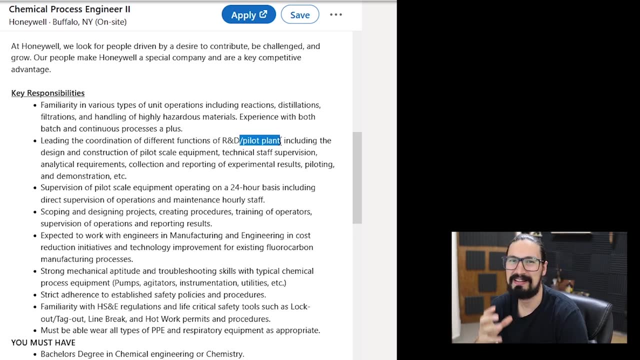 concept of leading. So whenever you see leading or main chief or actually something that says you, you're working towards that is a serious position, not just an assistant one. So great that you are going to be working with R&D and the pilot plant. This is by far one of the funniest places that. 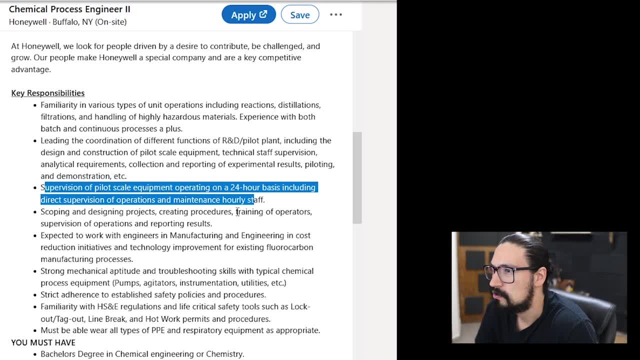 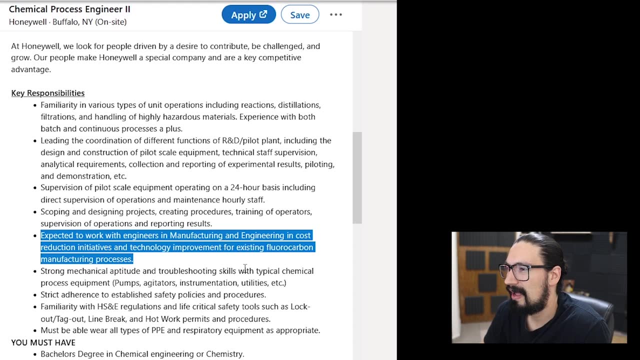 you're going to encounter because you're going to be working a lot with this pilot plant Supervision of the plant operating 24 hours. So that's also a classical one. on process engineering: Scooping and leaks: Once again this sounds major leaks. Expected to work with engineers in manufacturing. 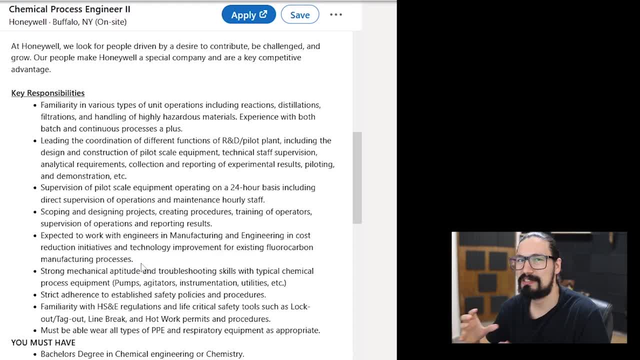 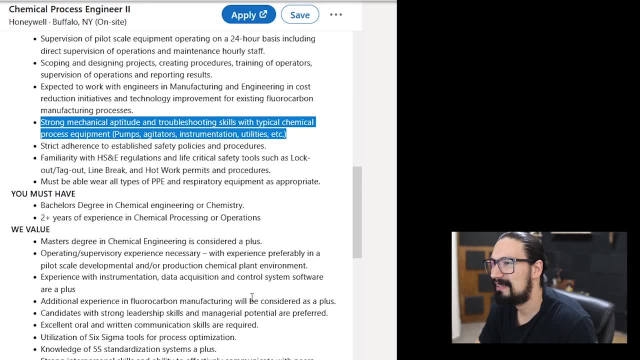 and engineering and cost reduction initiatives. So this is great. This is not only all about you and leading. it's also about working in a team. I really think this looks very promising. Strong mechanical aptitude and troubleshooting skills with typical chemical processes- Troubleshooting. 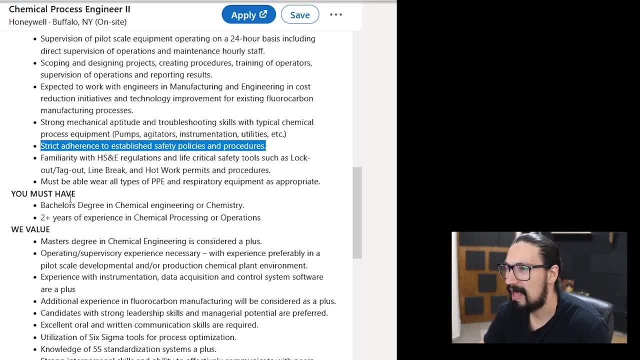 all the way, This is process engineering- definitely Must have bachelor degree in chemical engineering and two years of experience in chemical process operations. So interestingly funny to see that I specifically added entry-level job. I don't know how an entry-level job can have a requirement for two years of experience- My best. 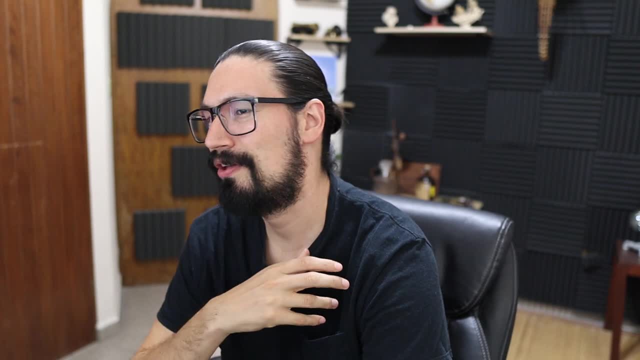 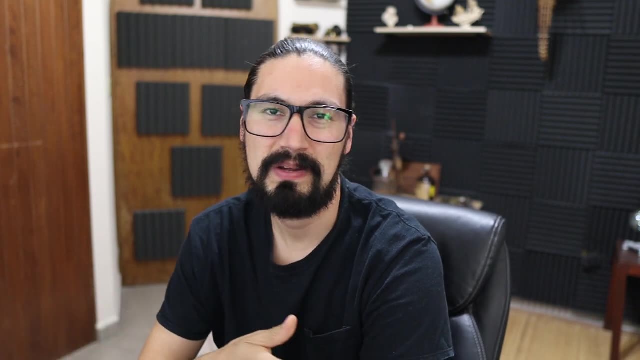 bet will be: guys, don't care, Just apply, It's going nothing going to happen. If they ask you, you can say whatever thing you think is actually worth, Maybe that you were in an internship or you had an R&D experience, or that you went abroad or whatever. 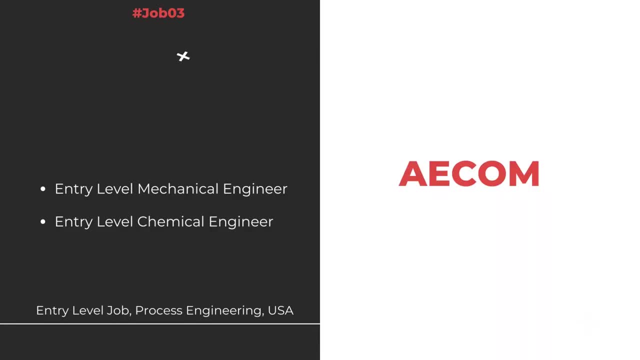 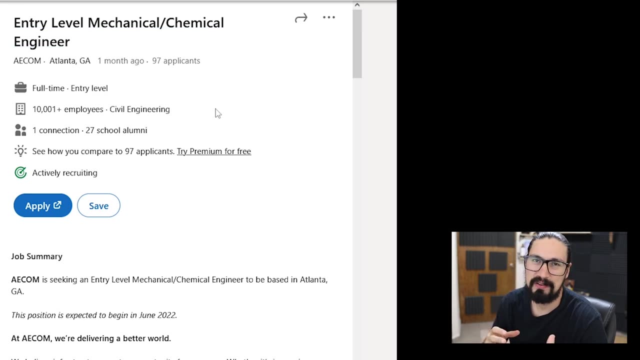 The important thing is to get that interview landed, Okay, so AECOM, Let's check it out. Entry-level mechanical or chemical engineer. So that's another thing that you can check out for is mechanical engineering. Maybe sometimes you can apply They. 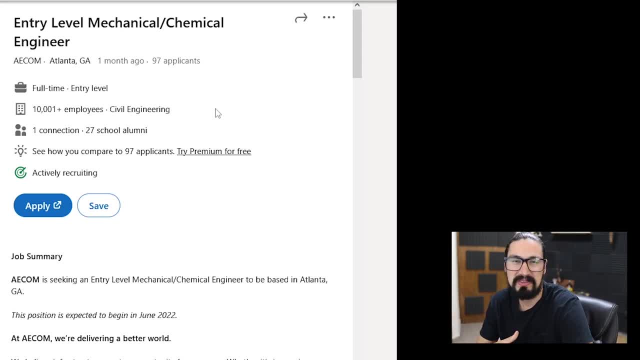 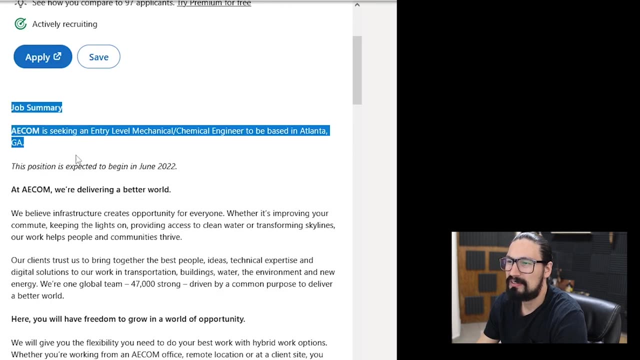 will not bat an eye. Maybe it's about actually implementing things, or quality or actual process engineering, Not that much into actual machine design or materials or so. So definitely also check out for that option. Okay, Quickly blah, blah, blah. Well, definitely, if you're actually interested, check this out guys. 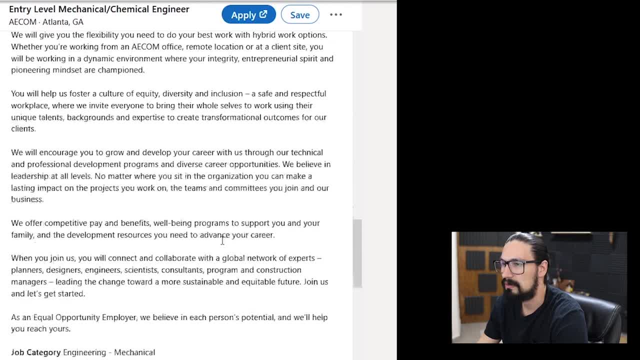 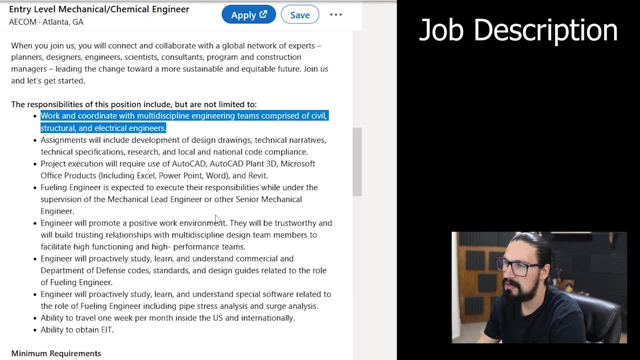 But what I want to do is the actual things that you're going to be doing. The responsibilities of the position include work and coordinate with multi-discipline engineering teams- Civil and electrical engineering- So this may sound much more towards mechanical engineering, but still stick to the job if you really want it. Assignments will include developing, designing. 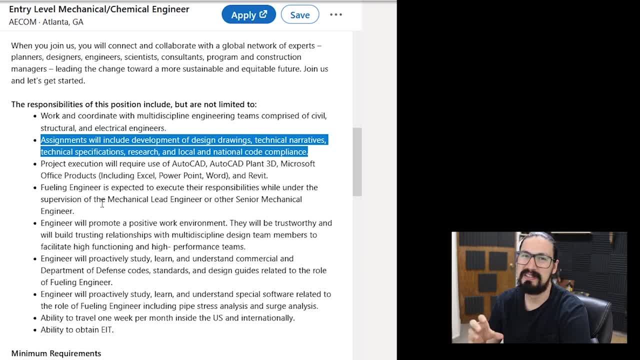 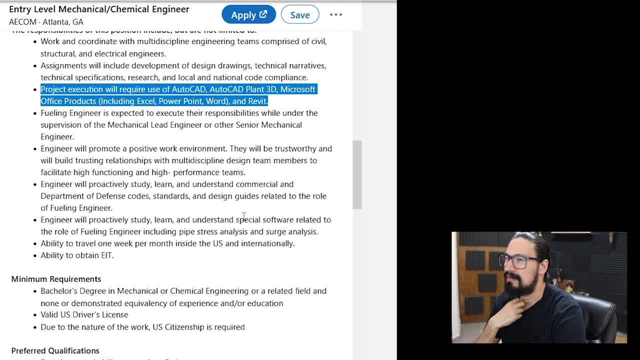 drawings, technical narratives: Okay, Once again, this sounds very, very like office work, assistant work. Project execution will require the use of AutoCAD. Okay, At least you're using an actual engineering tool: AutoCAD plan 3D. Once again, this seems much towards the mechanical engineering part, but doesn't mean that. 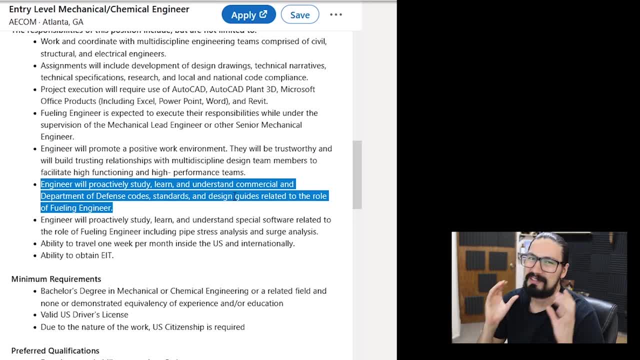 you cannot apply Productivity, study, learn, Okay. So this sounds very generic. In my opinion, this is most likely going to be someone working with a lot of paper, a lot of drawings, a lot of documentation, maybe A lot of documentation, So not that much actual work in the chemical plant. 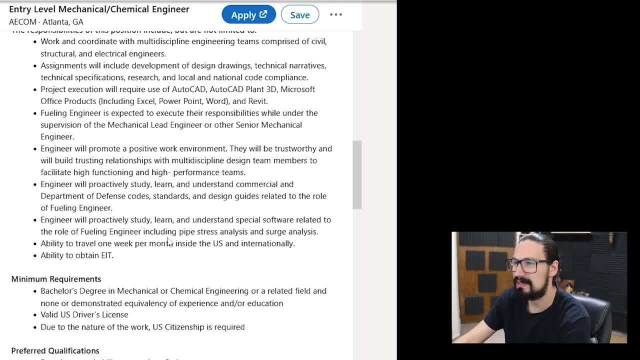 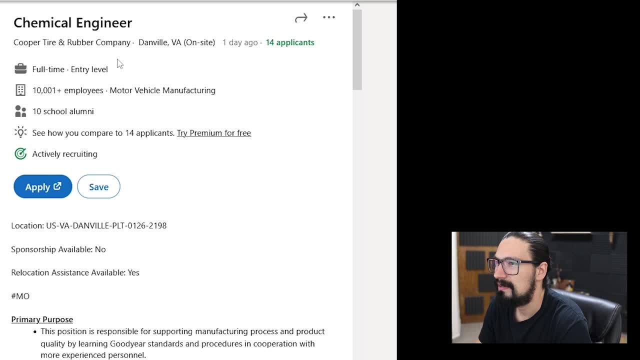 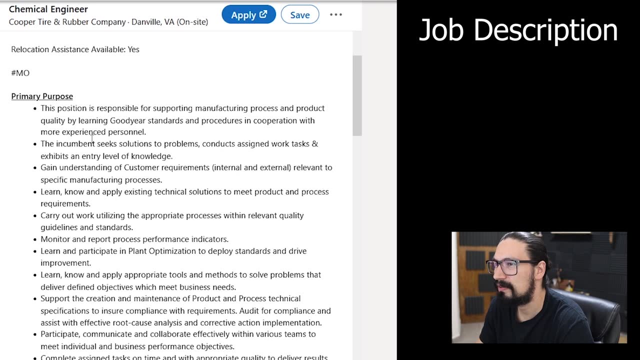 If there is any plant there, most likely you're going to be in the office. Okay, This one right here. Cooper Tire and Rubber Company. That sounds very chemical engineering-ly. This position is responsible for supporting manufacturing process and product quality by learning Goodyear standard. Okay, Very abstract. The incumbent six. 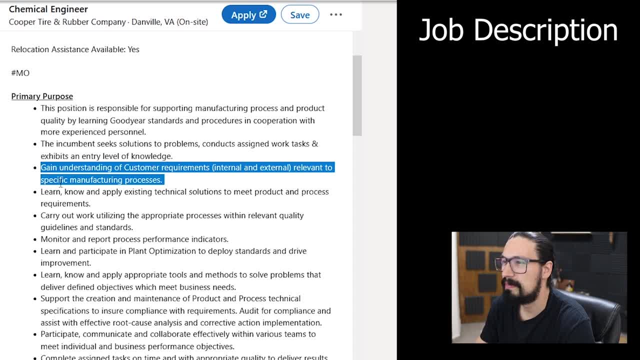 solutions to the problem. Okay, Customer requirements, That's great. Internal and external. So I really prefer when you see external customers, because that means that you're actually working with other customers or clients, Not that much into the whenever they say internal customers. 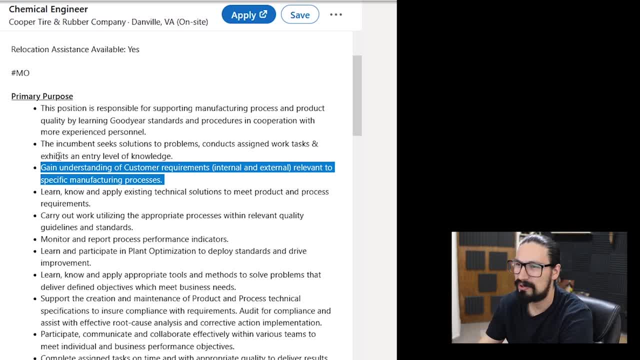 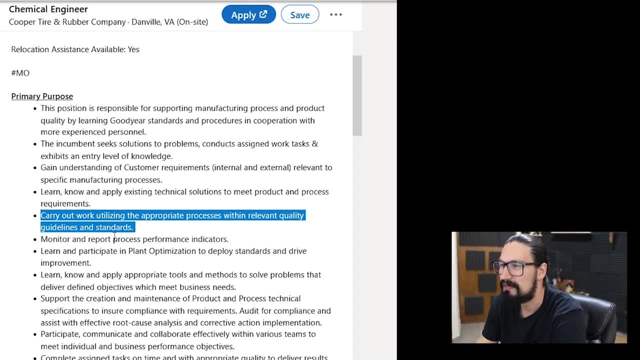 it's actually just people working with you guys, So this may be tricky. This is a very generic description, So actually these are common tasks of everyday engineering. Monitor and report process performance- Okay. KPIs Learning and participating in plant optimization to deploy standards- Okay. 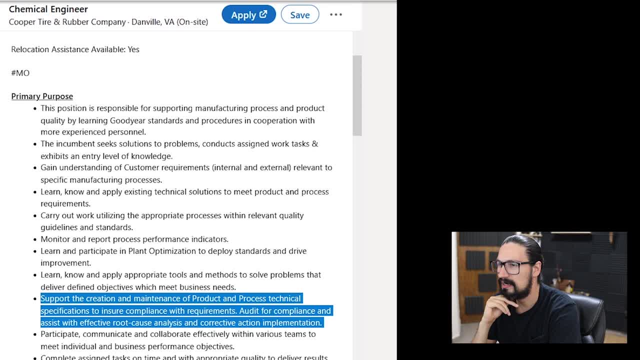 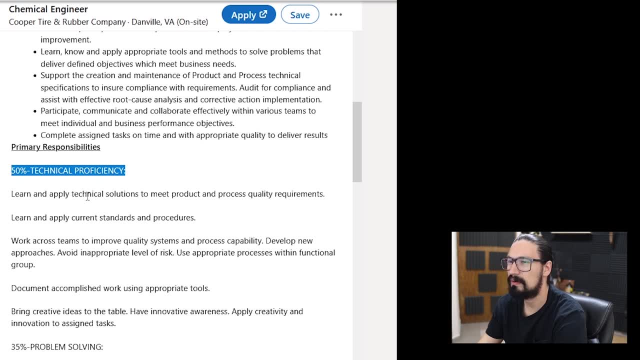 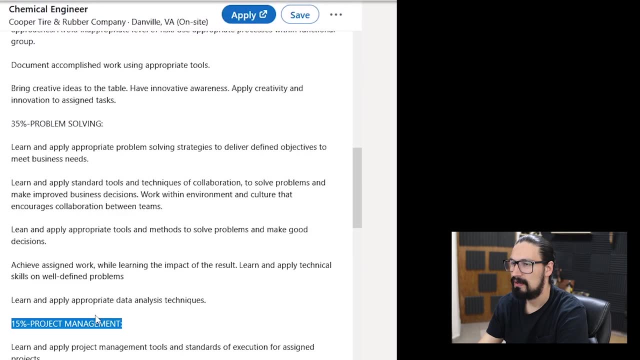 Support the creation and maintenance of products and processes. technical specifications: Okay, So responsibilities. 50%. technical proficiency- So actually knowing about technical solutions to solve problems- Okay. Problem solving and project management: Okay. Now guys, project management. may sound great that you're going to be working with an actual project, but, to be honest, 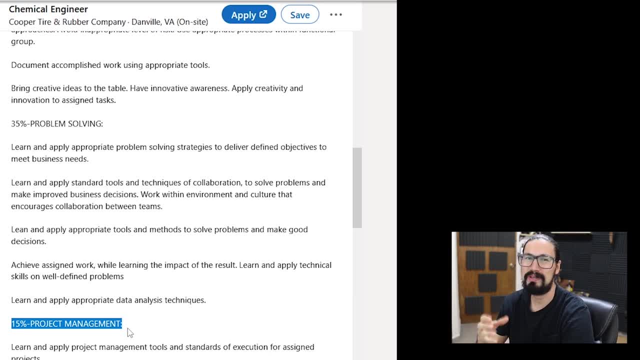 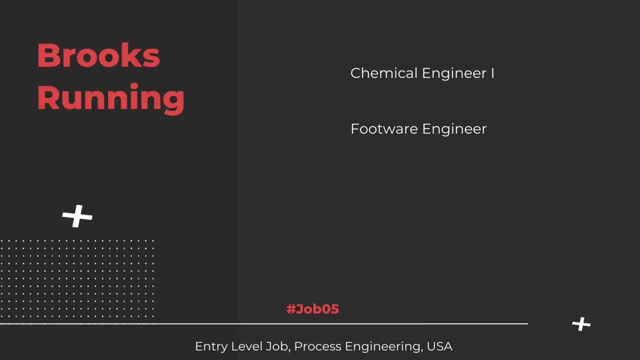 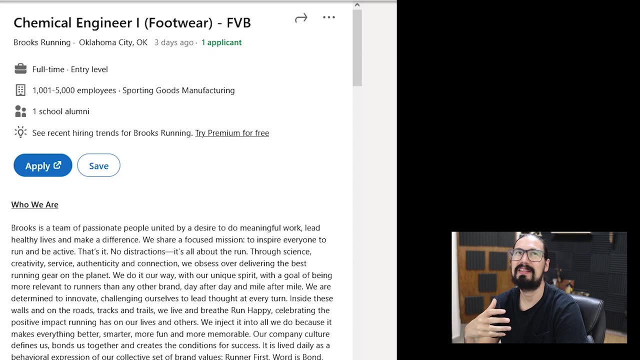 project management many times means that you are just going to need to work with your scheduled time and your own resources. Let's go and check out this one right here: Chemical engineer. one footwear. I'm very looking forward towards what. what is that that they need? a chemical engineer, Most likely. 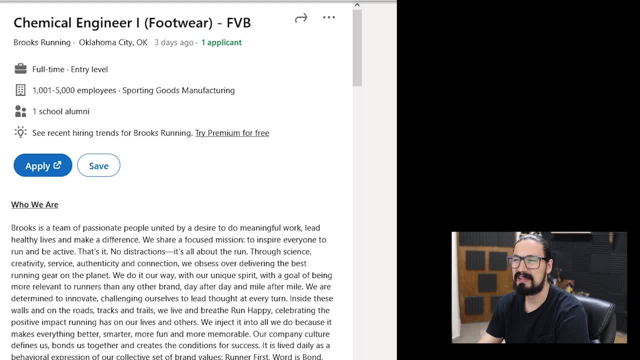 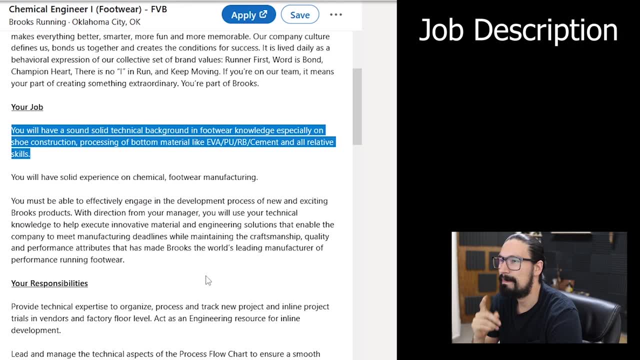 because of the polymers they're using in their footwear, or maybe the textiles- I don't know, Let's check it out- Or maybe even the production. Okay, Your job. You will have a sound, solid, technical background in footwear knowledge. So that's great. They already promising you to train. 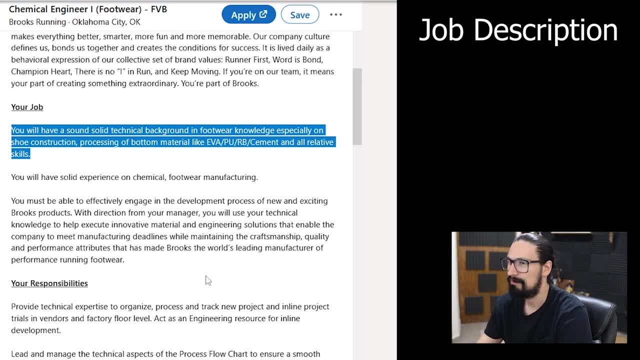 you in footwear industry. So if you want to develop that, that's right, Especially on the show construction processing of bottom material. So essentially we're talking about working on this part of the footwear, So that may be great. I'm not looking forward. If you're looking for polymer, 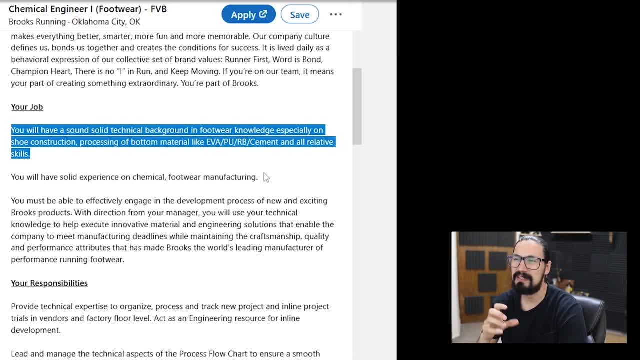 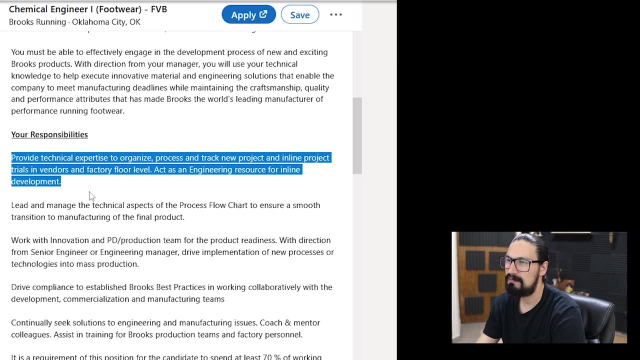 extrusion or that. this may not be the case. Maybe it's already constructed and you're just manufacturing or Just pasting it and working with it, So let's see what. what else we can rescue from here: Provide technical expertise to organize, process and track new projects. Okay, Sounds great. 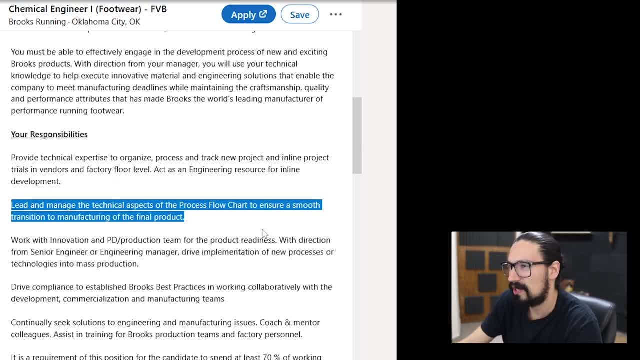 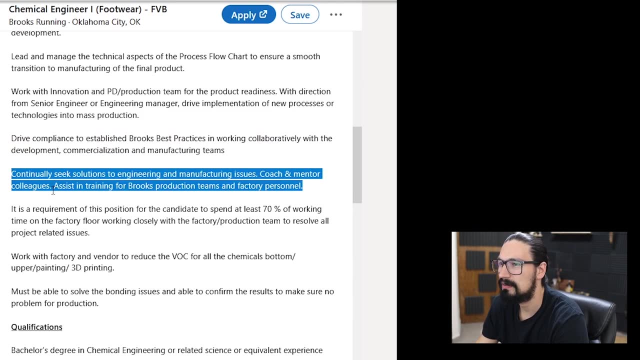 Lead and manage technical aspects. process flow chart to ensure smooth transition to manufacturing. So essentially, this is process engineering 101.. So you have a plan and you need to implement it in the actual manufacturing Work. with innovation Drive complex. Okay, Continue the. 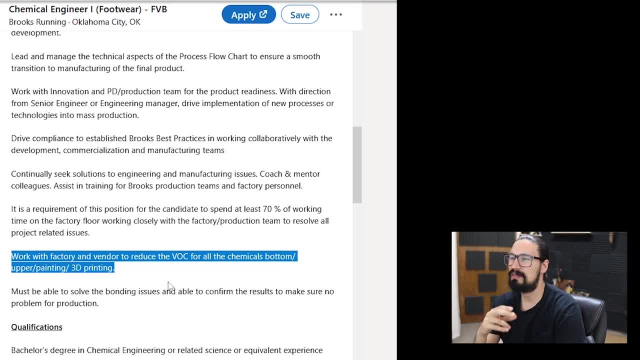 process. Okay, I like this work with factory and vendor to reduce the VOC, which is essentially the volatile organic material or compounds, uh, which sounds very non-healthy or hazardous while upper painting and 3d printing. So, uh, if you're into shoes, this may be very promising guys. If 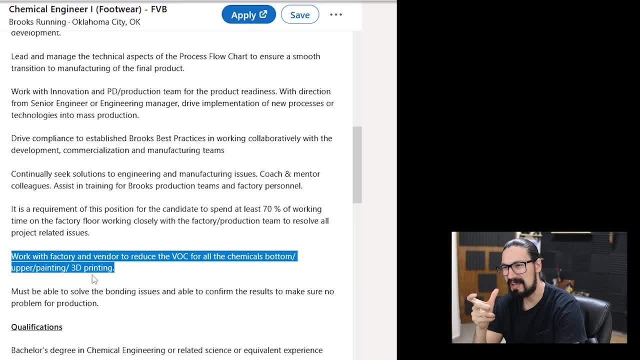 you're into very chemical materials. this may not be the case, but this may be an entry level position, So you get used to shoes or maybe the actual polymer 3d printing. This can bring you to other places, So definitely worth checking out this job. 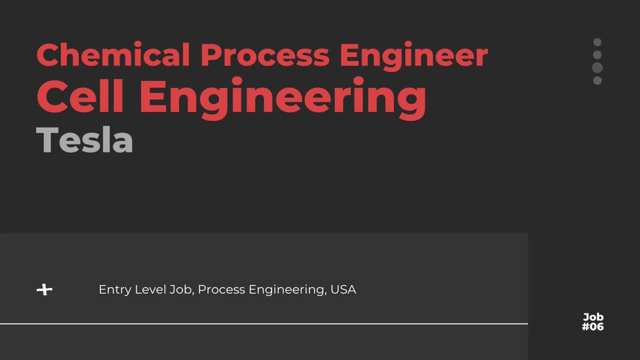 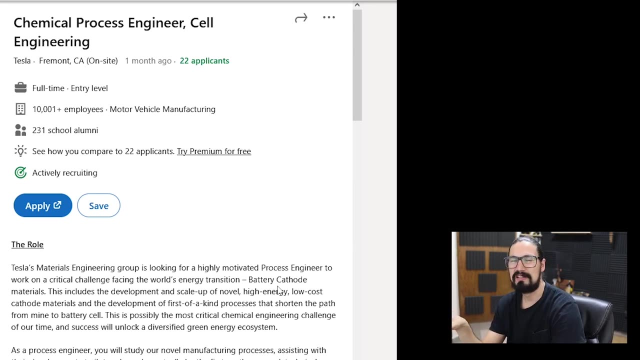 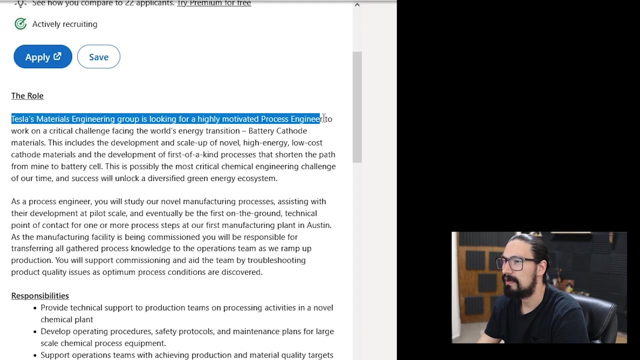 Let's go to this one right here, which I'm pretty sure, guys, that you're interested. And of course, we got Tesla cell engineering and not we are not talking about biological cells, We're talking about electrical or electrochemical cells. The role Tesla material groups highly motivated. 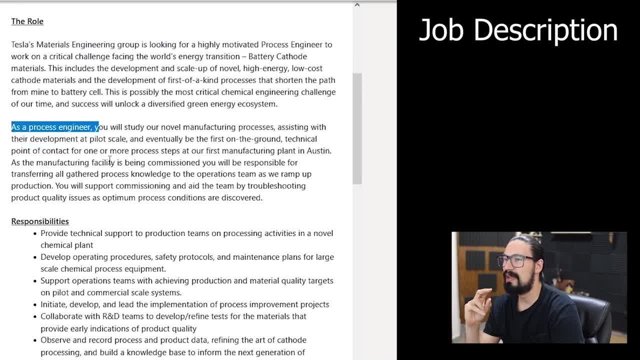 Okay, Blah, blah blah. As a process engineer you will study a novel manufacturing processes. Okay, Become the first on the ground. So that sounds very process engineering. I love that in the Austin plant is the very first. like big city- well, Oklahoma city, but Austin like. 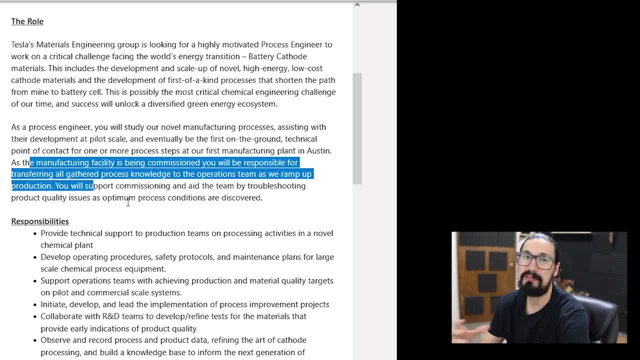 an actual nice city worth checking out if you're into big cities, if you are irrelevant or you don't care that much. And of course we're not checking out the salaries, guys right now. we should expect something between 60 to 80 K overall. Mmm Responsibilities: provide technical support. 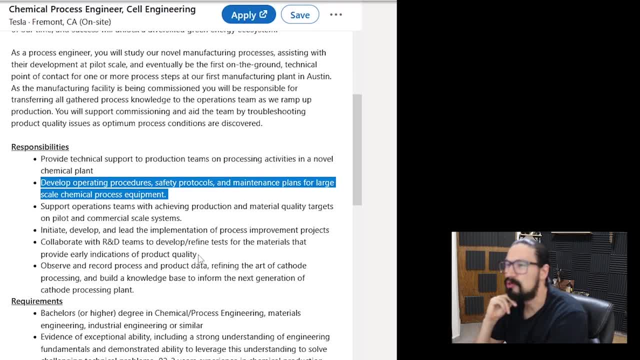 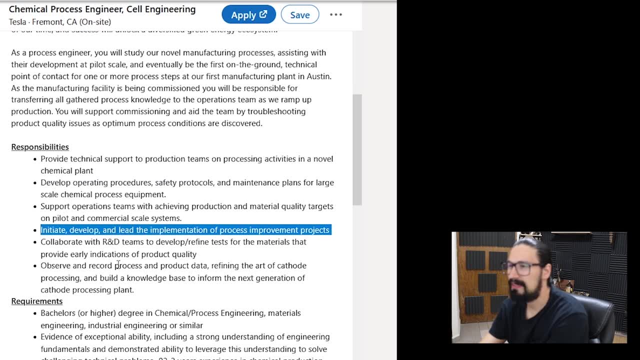 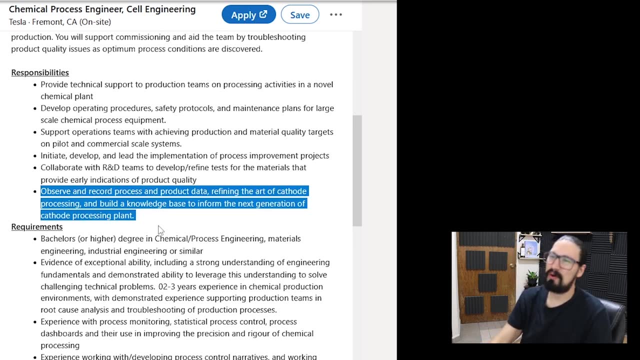 Okay, classical one: develop operating procedures- okay, that's also classic, i think. process engineer, you will need to actually implement stuff: initiate, develop and lead implementation. collaborate with r&d, research and development. okay, to be honest, this sounds very, very broad. it does not state something technical. are you going to be working a lot in the chemical plant, in the pilot plant? 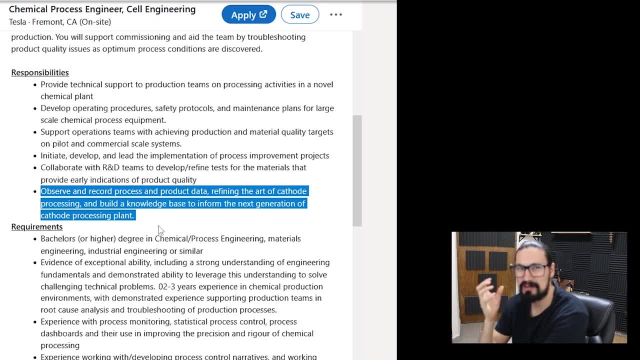 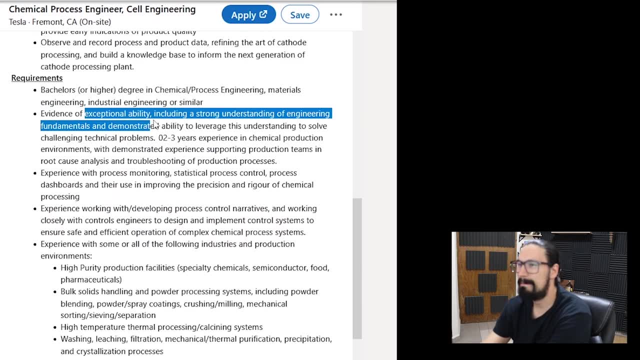 in the manufacturing plant. are you going to be studying the actual batteries, the actual cells, or are you going to be producing them? it's not quite straightforward: exceptional ability, understanding engineering fundamentals, experience with process monitoring- once again, entry-level job. how do you expect to have process monitoring experience other than being in a co-op or 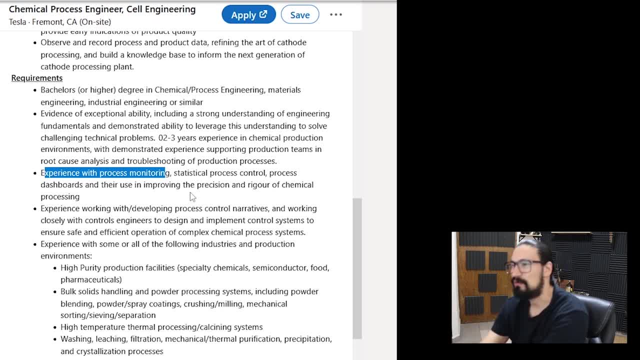 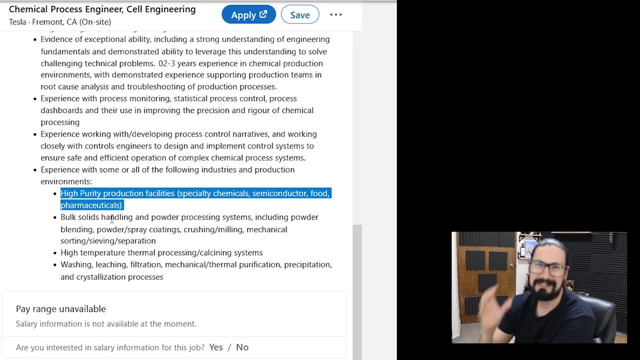 internship that have specifically that it's kind of hard to do this statistical process control so, honestly, it's way easier to get a one-year job related towards process engineering and say that you have the experience okay, working with high purity production facility. yeah, this is not an entry job, guys. this is definitely looking for someone that maybe between one to three years. 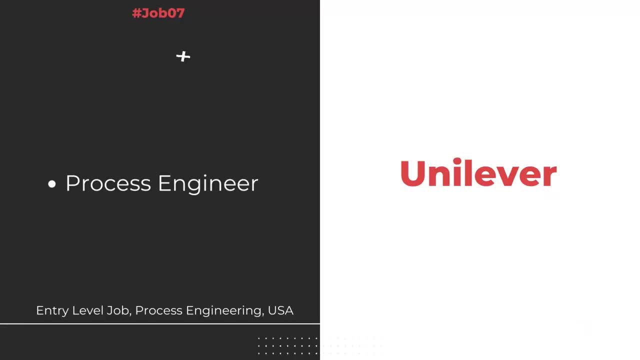 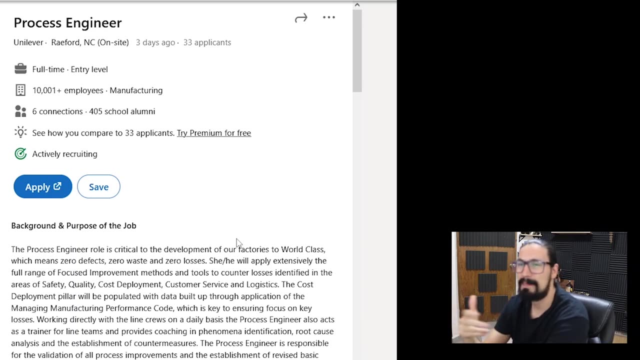 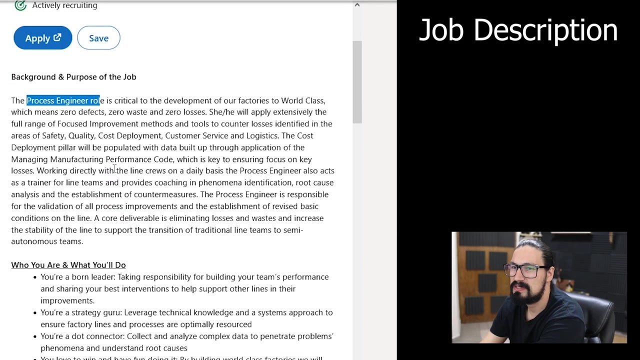 working in a process industry already- Unilever. I think this is going to be the last one that we're going to check out. definitely, Unilever is one of the top companies. chemical companies are only. they should be one of the best chemical companies to work in. so let's see it out, okay. so process: 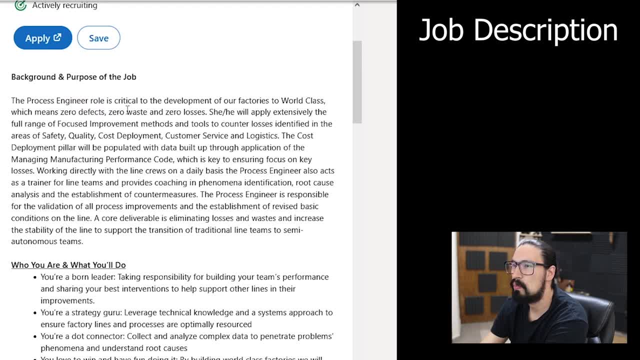 engineering, all is two okay: zero effects, zero waste, zero losses. it's almost impossible. you cannot have zero defects. this is like the definition of six Sigma. by definition, you have defects, zero waste- impossible in any process. engineering, there's always waste and zero loss. I don't know what they mean with that, but anyways, working directly with the line, 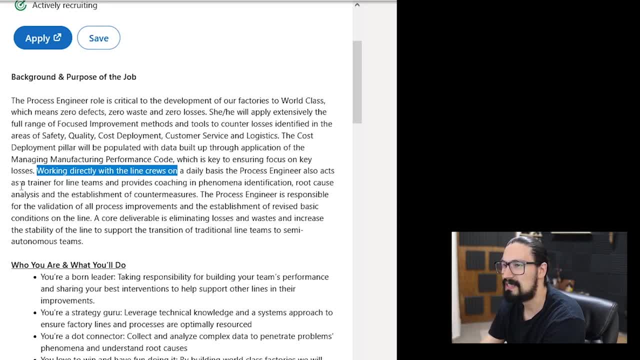 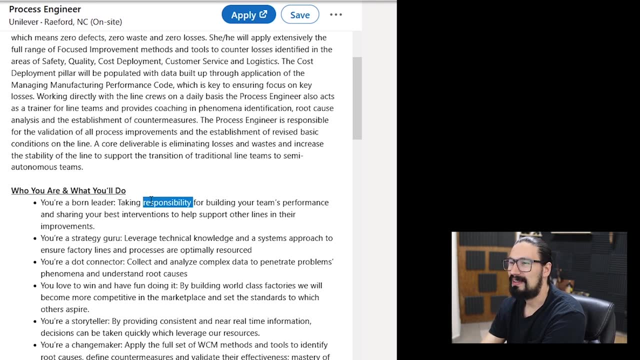 crews. so, on the daily basis, presenting also acts as a trainer. okay, you're going to be working with people. is responsible for validation of process. okay, let's go to. who are you and what are you going to be doing in this company? you are a born leader. okay, I like the way they approach this, of course. 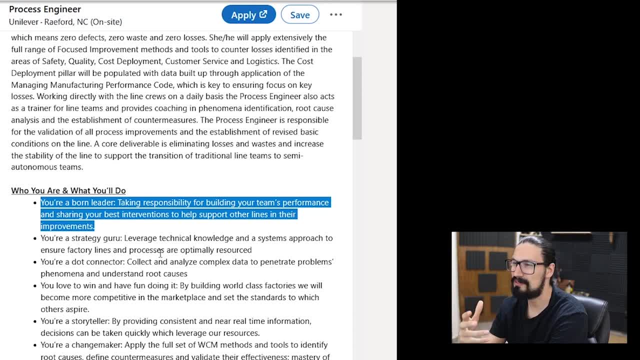 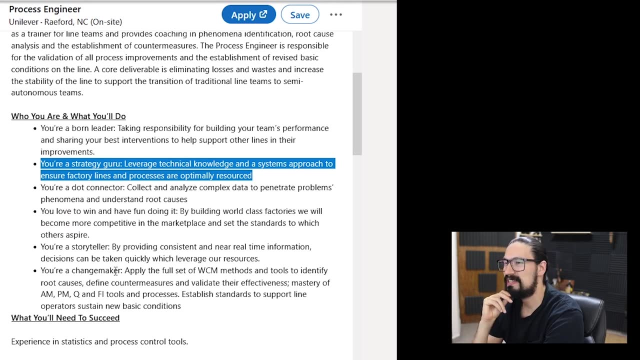 companies are looking for leaders that can be paid so they can carry the company on taking responsibility for building your team's performance and sharing your best interventions to help support other lines in their improvement. you're a strategy guru. leverage technical knowledge and systems approach to ensure factory lines and processes. 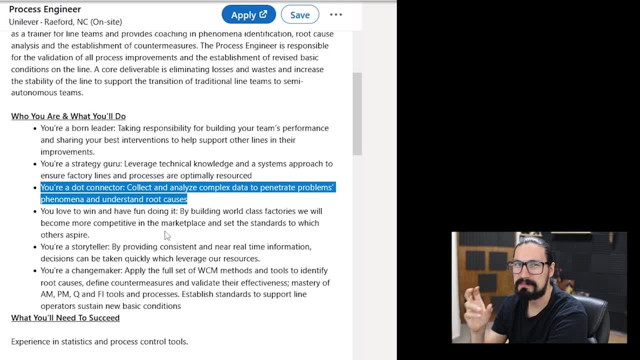 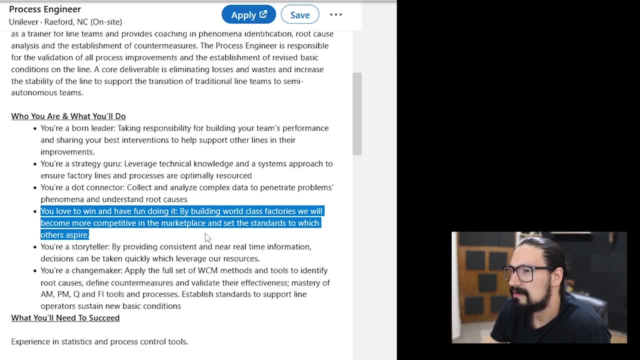 are optimal. you are a doctor connector by definition. a process engineer must be a dot connector. that's all the way true. collect and analyze complex data to penetrate problems, phenomena and, of course, solve them. you love to win and have fun doing it. building world class factories, we will become more competitive in the marketplace. okay, you are a storyteller by. 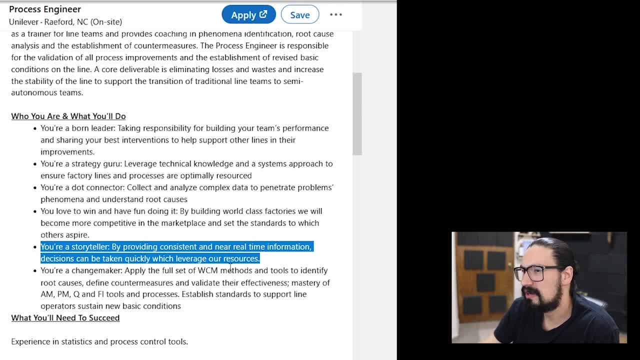 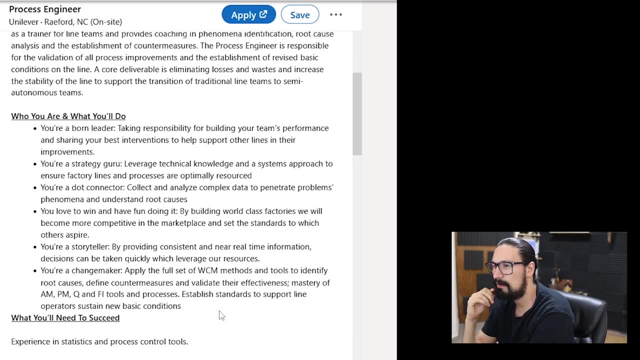 providing consistent and near real-time information, this decision can be okay. definitely, this has not tense at all. I don't know why, storyteller, but hey, they are trying to make like interesting this position. you're a change maker. apply the full set of the WCM methods. what you will need: experiencing statistics and process control once. 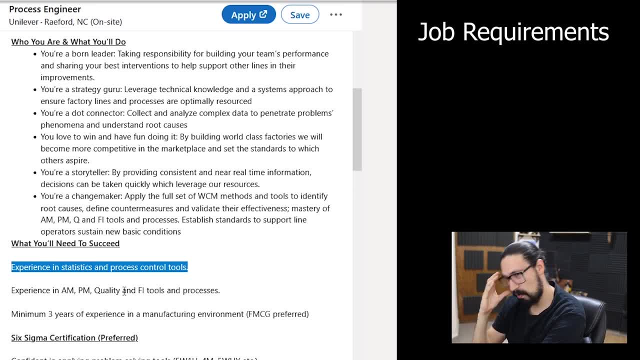 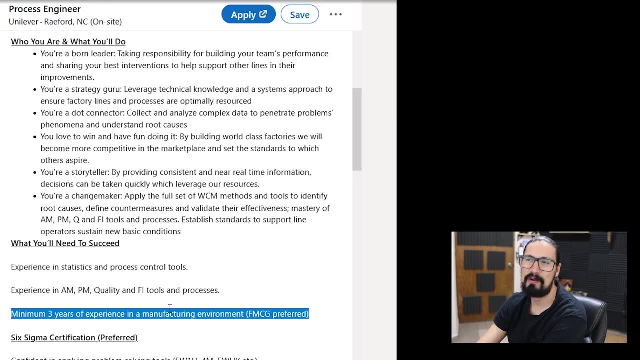 again, this is supposed to be an entry-level job. I don't know why are they doing this? well, I know they want to get people with experience, but see them in the entry level uh range of payment or salary. minimum three years of experience in manufacturing environment- definitely. I don't know why they filter in the entry level jobs. 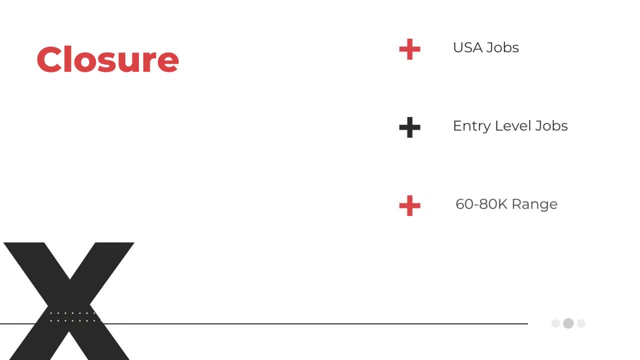 and that's it, guys. this is what I wanted to show you guys: how you can search for chemical or process engineering jobs, depending where you're looking for. right now we search in the US, the whole USA, but I'm pretty sure that if you live there, or maybe you want to move there, you may want to. 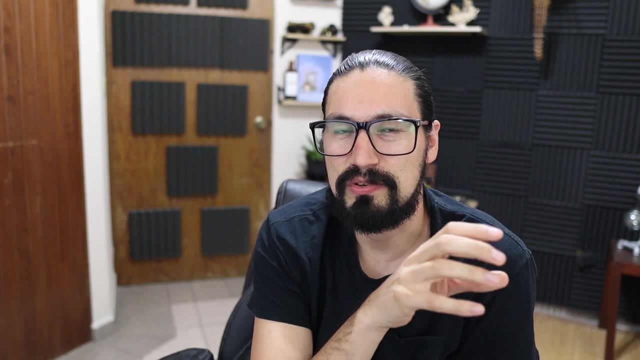 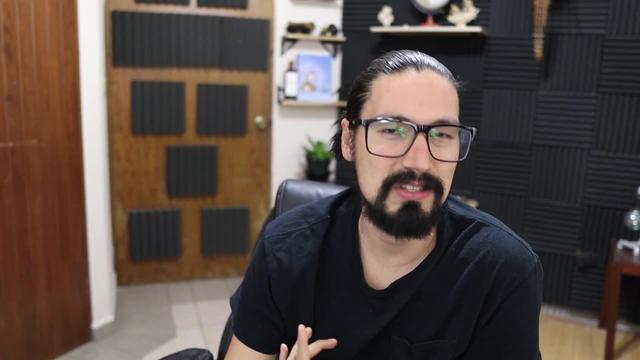 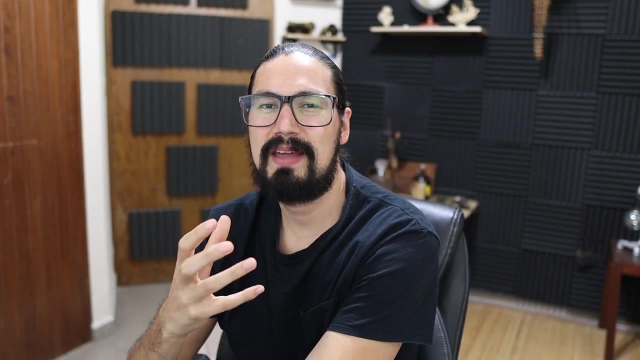 search per state or per city. maybe going and search for California or going for Texas, maybe something in the New York or Boston area, the Chicago area? that's up to you, guys, but at least right now you know how to do it. and, more importantly, guys, what I want you to get from this video is that there are many jobs. 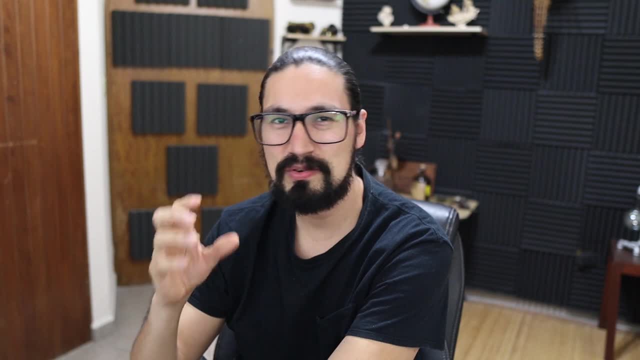 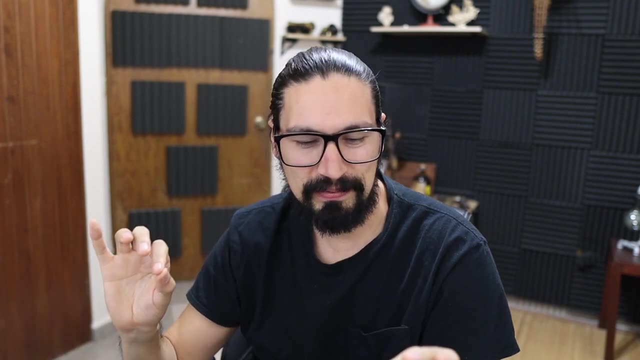 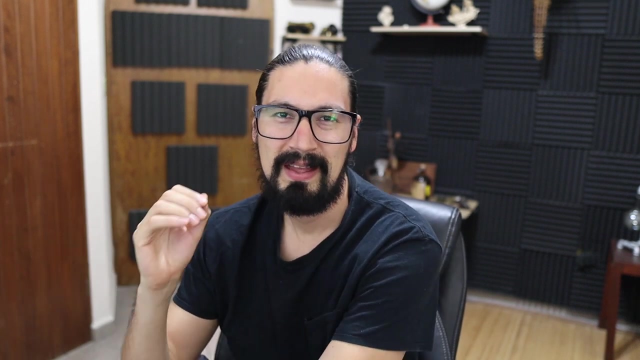 that sound great but are on paper, ones that you go there, work there, you will see and read it and you will be able to maybe allocate and say, okay, this first point is okay, I'm actually doing that, but many times a lot of this is just nonsense. documentational ones, the